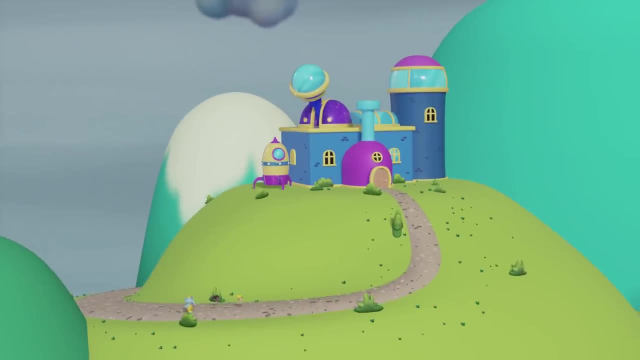 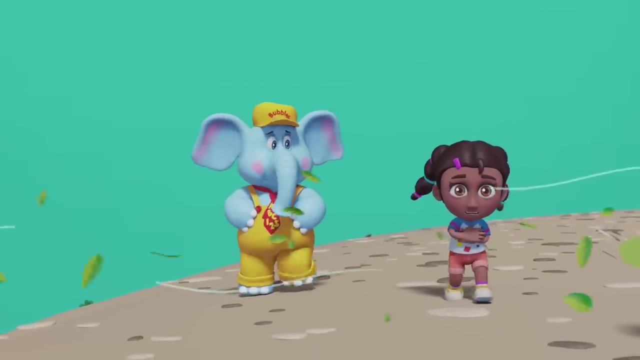 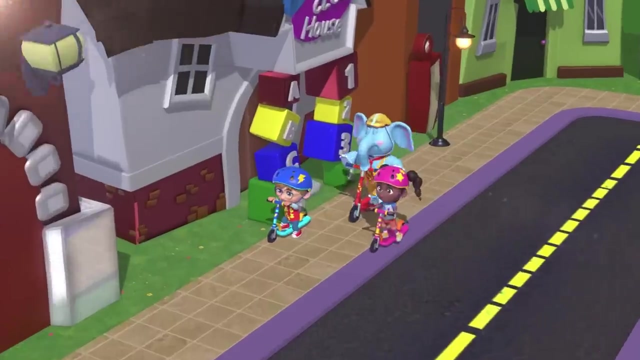 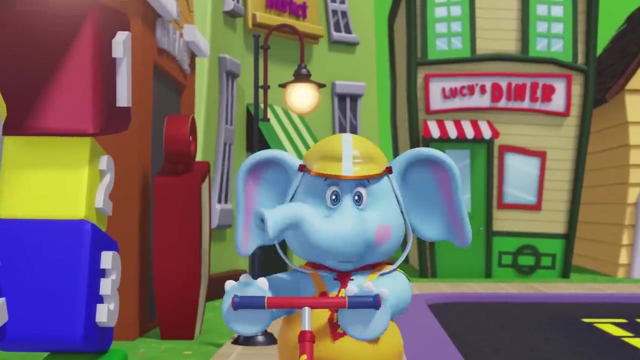 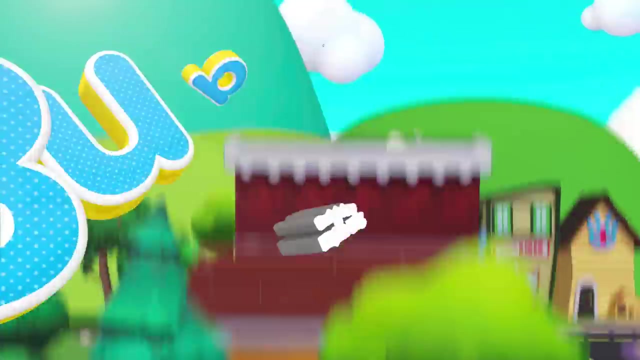 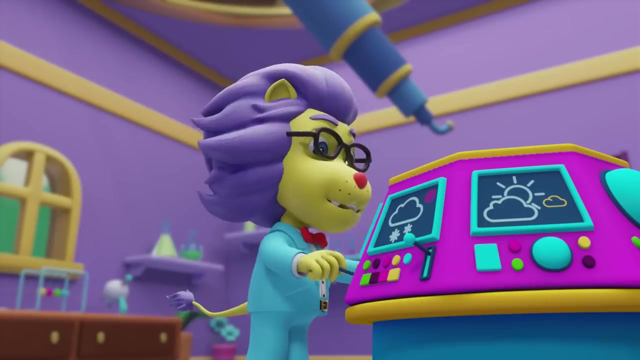 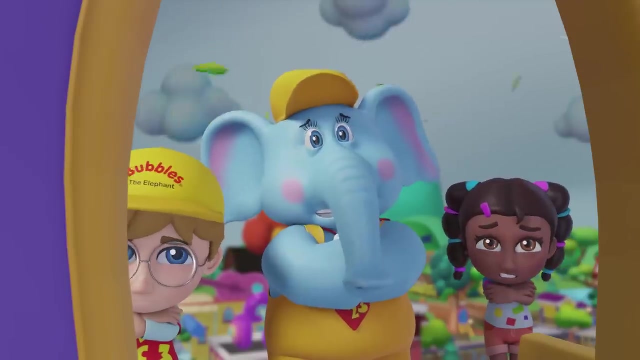 It's a beautiful day to come and play and learn a thing or two With Bubbles and Friends. the fun never ends. We're ready. how about you? Bubbles and Friends Weather Machine. Hello Hi team. Oh, come inside, it's warm in here. 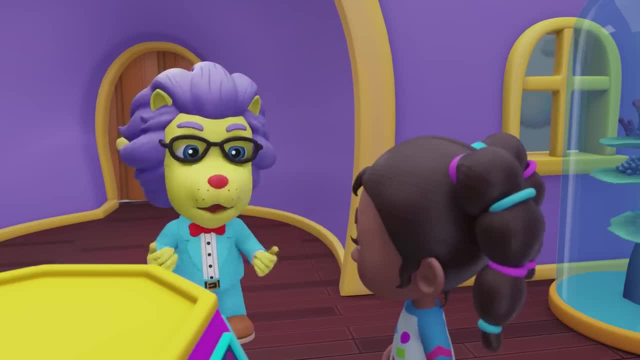 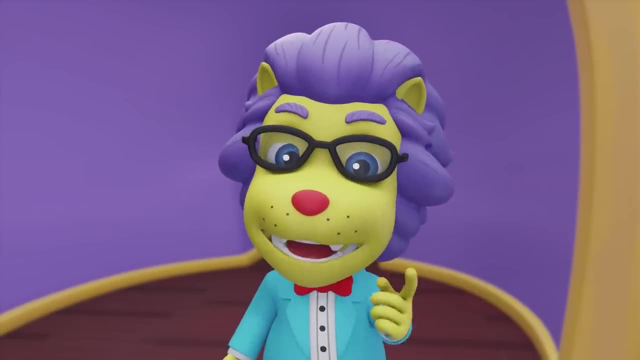 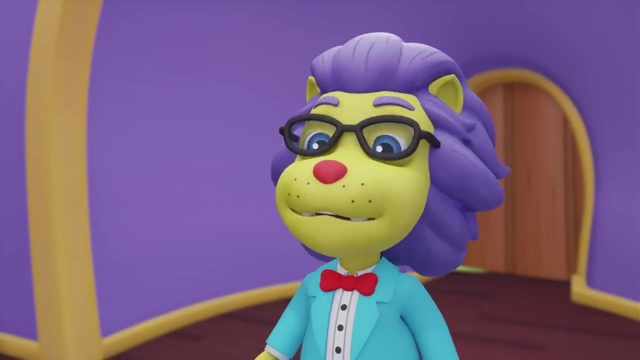 No scarves, No jackets. You need to stay warm in this weather Weather. The weather is how the sky and the air feel outside. The weather today is windy and cold. Hello Team, do you want to try out my weather machine? 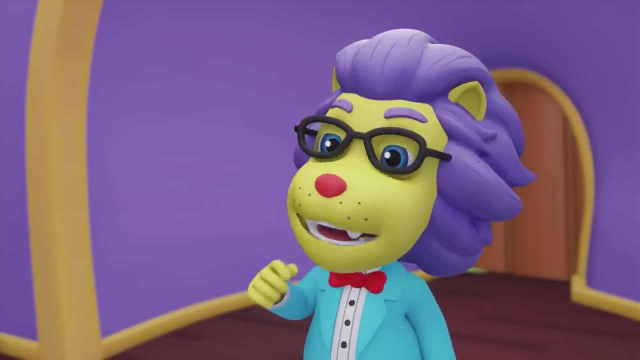 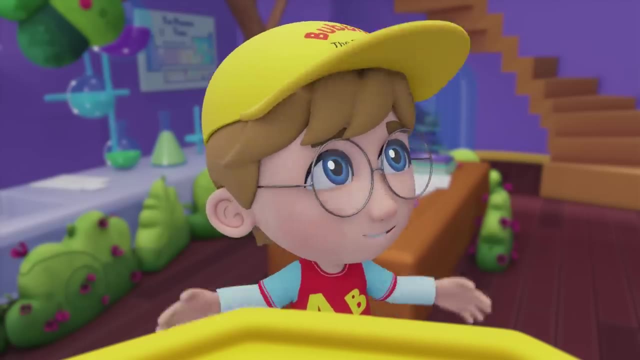 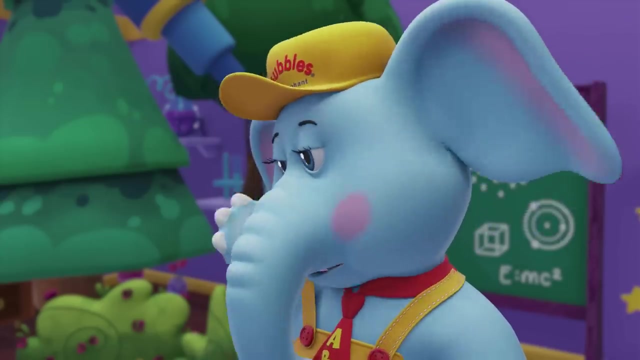 We can explore different types of weather and see how they feel. Yes, Yes, Whoa, This is amazing. It's so sunny. There are no clouds in the sky, Phew, it's super hot. Usually on sunny days, the temperature goes up, so it's warmer. 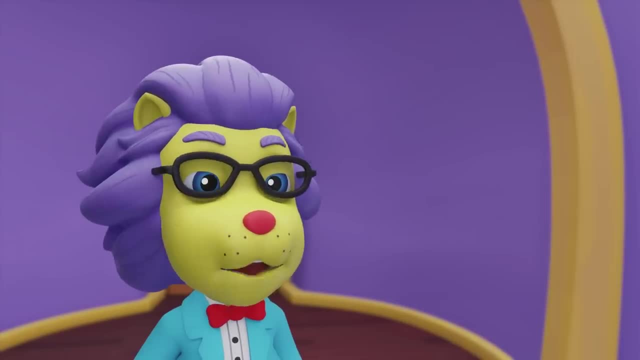 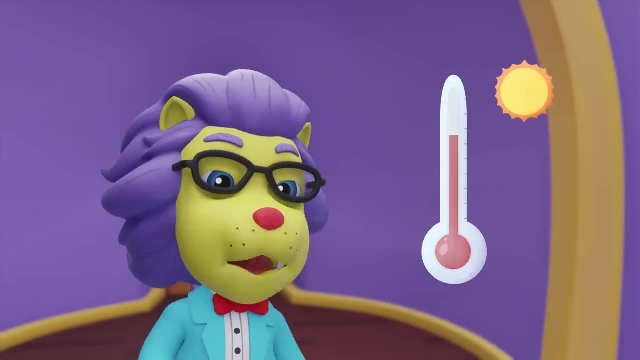 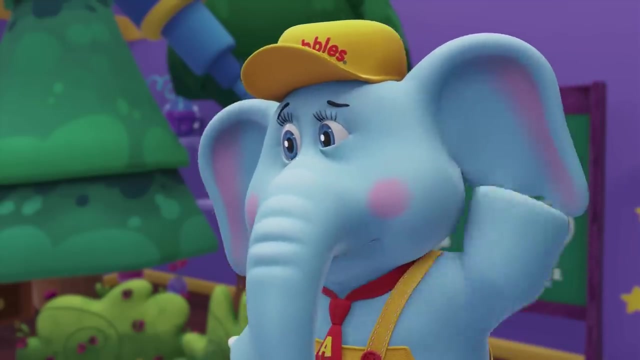 What is temperature? Temperature tells you how hot or cold the day is. When the temperature is high, it is hot, And when the temperature is low, it is cool. Hmm, the sun feels so nice. Uh-oh, I didn't bring any sunscreen. 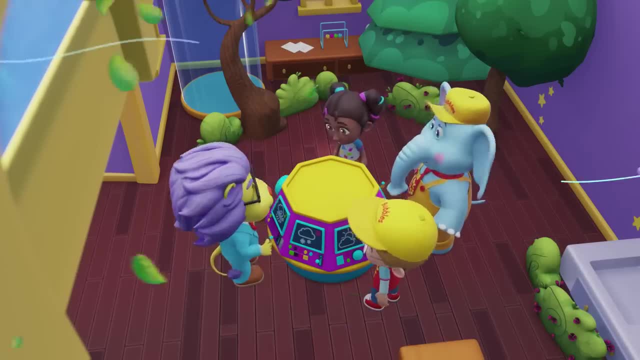 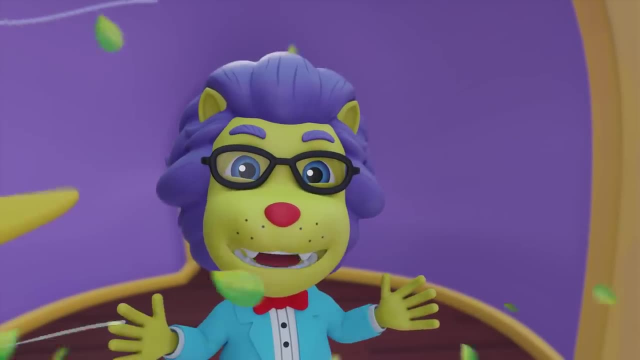 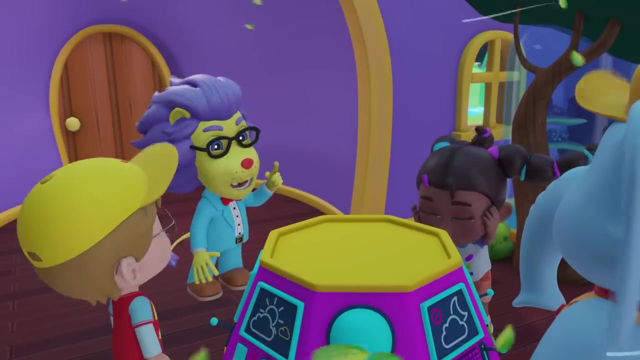 That's OK. No wind: Wow, Look at those leaves floating. This is a windy day. The air moves really fast like a fan blowing on us. Even if it is sunny, it can feel a bit cool because of the wind. 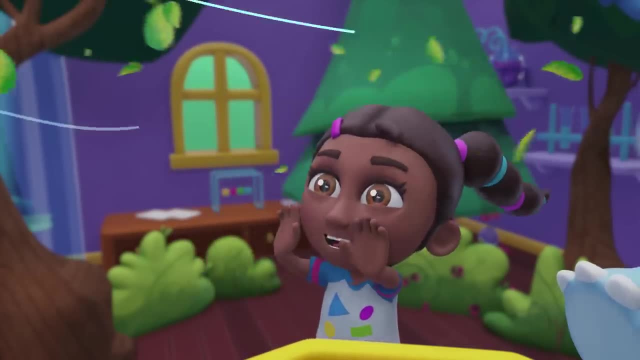 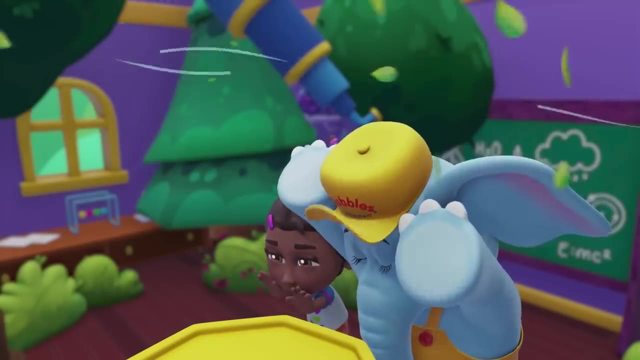 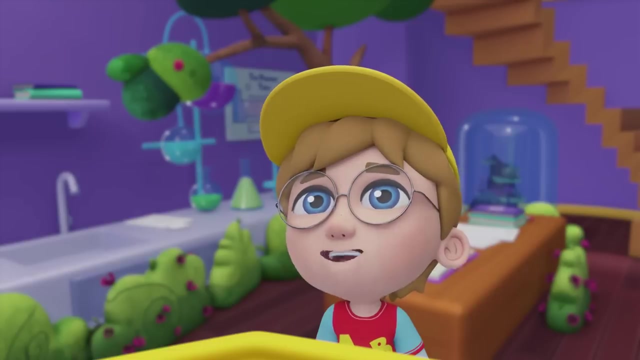 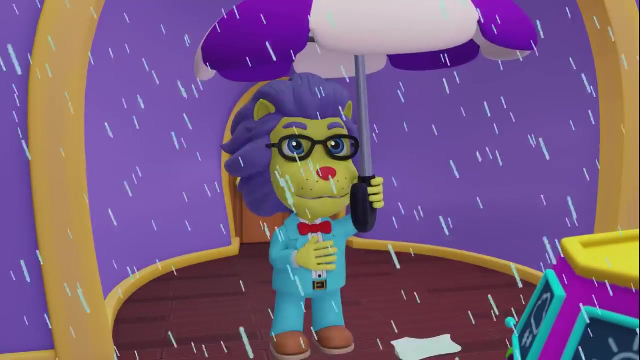 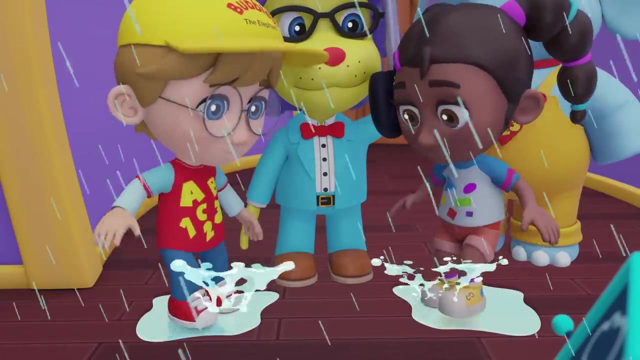 I can barely walk. The wind is pushing me. Hold on to your hats. Look how dark they are. now It's so gray and gloomy. Watch out for the rain, Just in time. This is fun On rainy days: the clouds cover the sun and it gets gray. 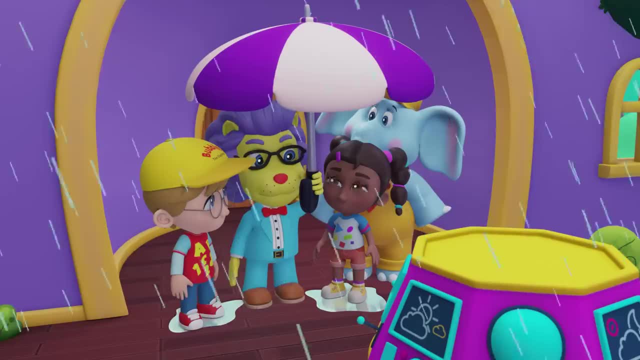 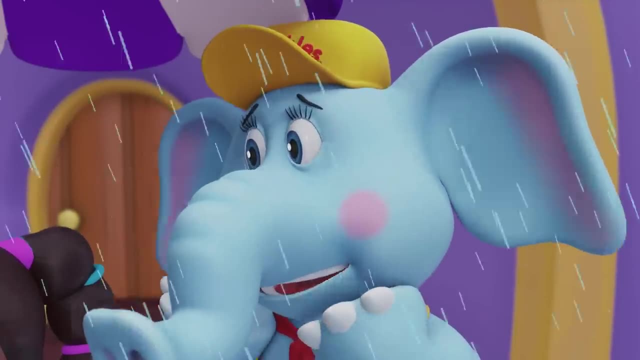 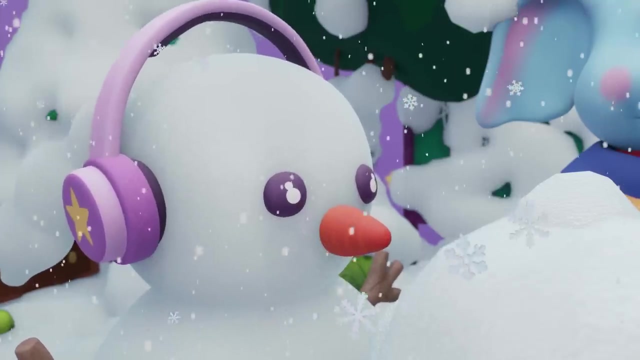 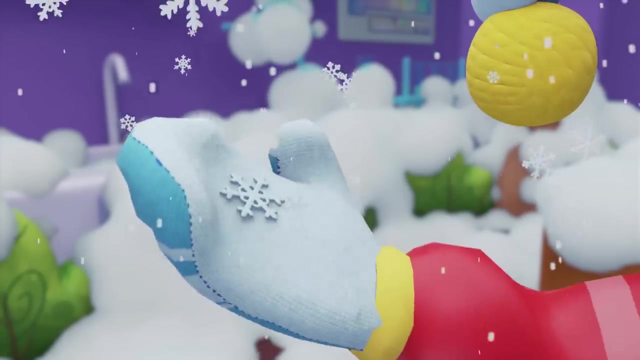 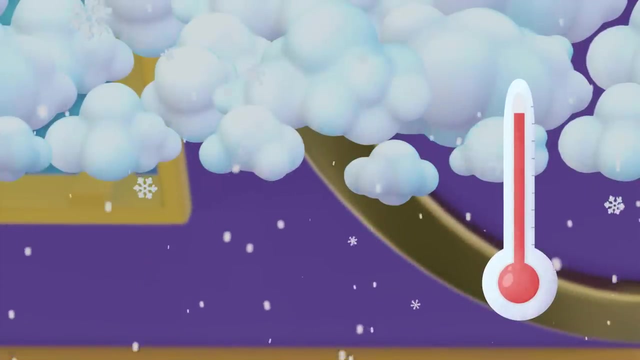 And dark And everything gets wet. of course, Time to leave. Yes, please. It's cold and snowy. Snowflakes. It melted on my hand. Ah, that's because snow is, It's made of water. When temperatures drop, it can freeze and turn into snow. 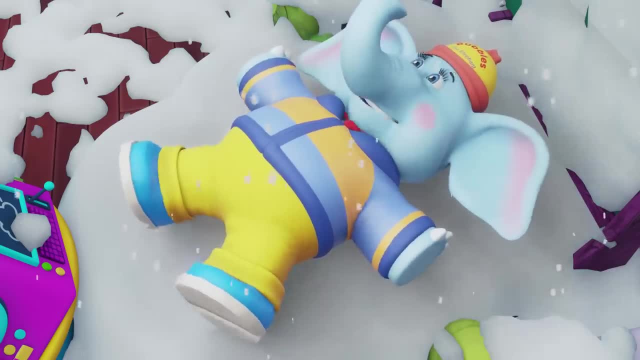 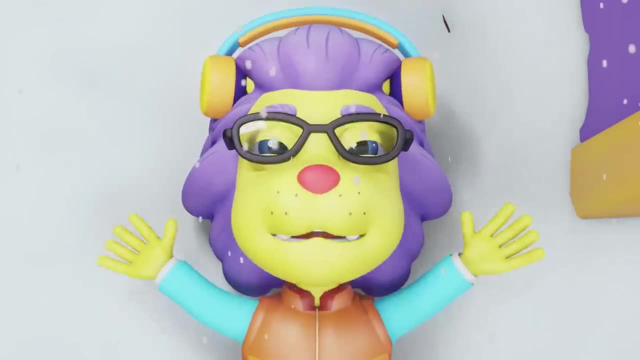 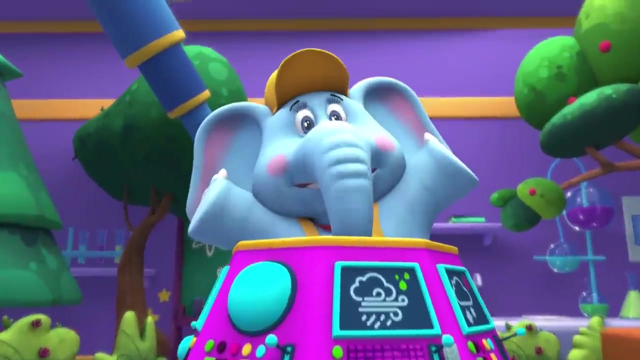 It's like ice, only softer. It's soft and wet and cold. Whoa See, all weather is fun in its own way. On the sunny days, we're on the move Under the sky, we dance so smooth. On the rainy days, we splash. 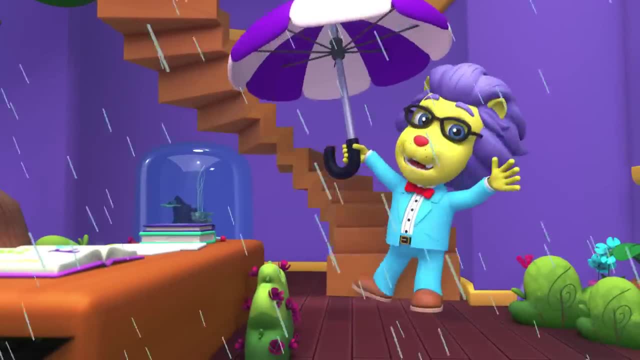 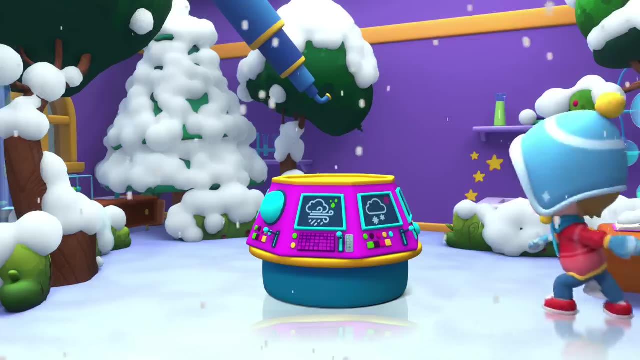 In pain In the puddles. we dance the great days away. When we feel the windy vibes in the air, We sing along with the breeze in our hair. Almost no, we snowy winter days that shine, We glide on the ice and we feel so fine. 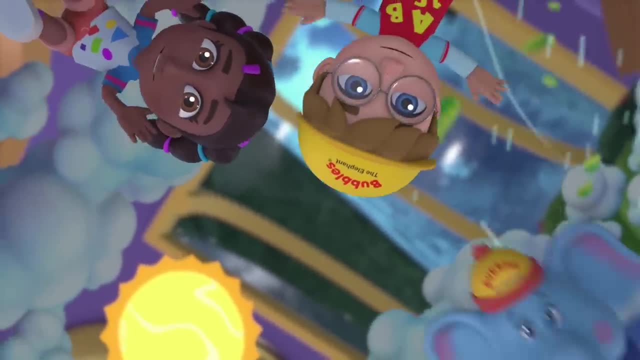 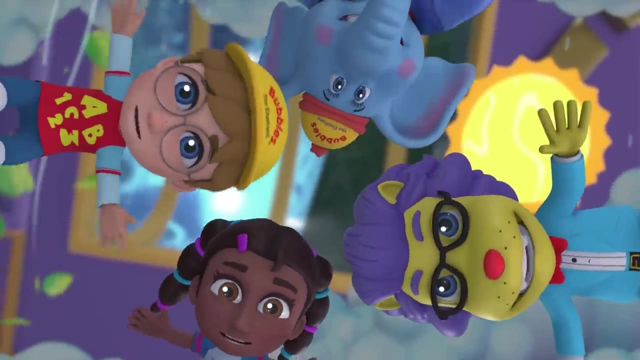 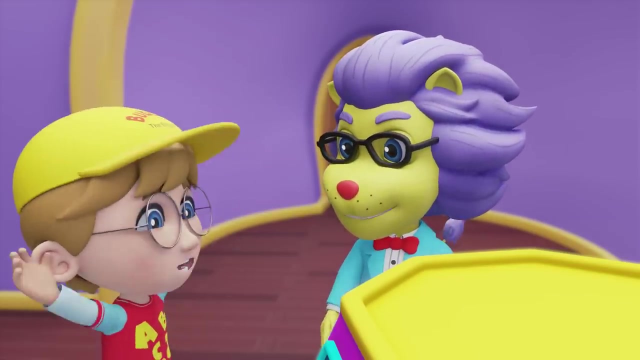 Rainy or sunny, we play along In Happyville, where we all belong. Windy or snowy, we play along warmth In Happyville, where we all be-yum. That was so much fun. I loved the weather machine. 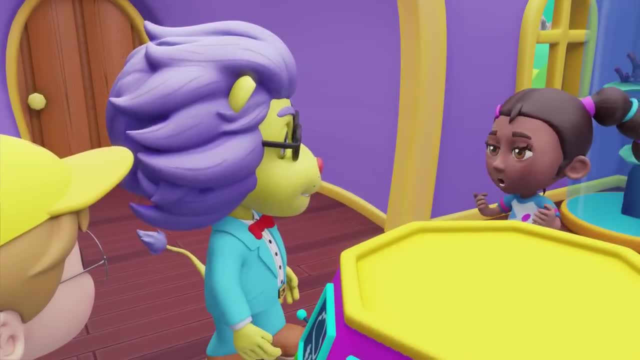 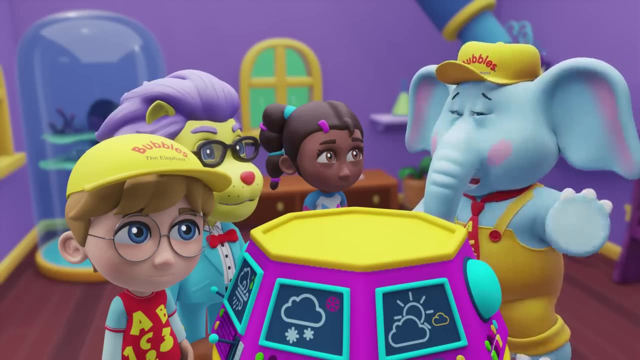 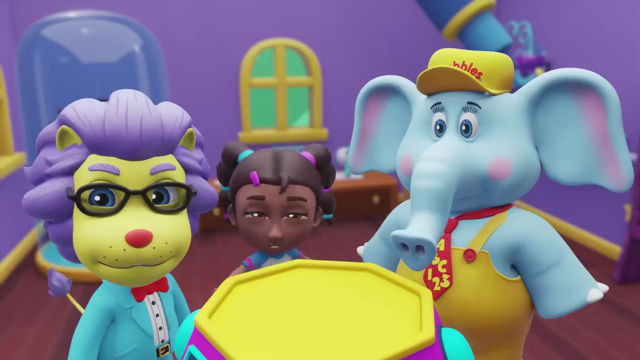 Now I think my favorite weather is All of them. Thank you so much, Lionstein. You are welcome team. What's going on with the weather now? It's raining. Look at all those puddles, Let's go jump in them. 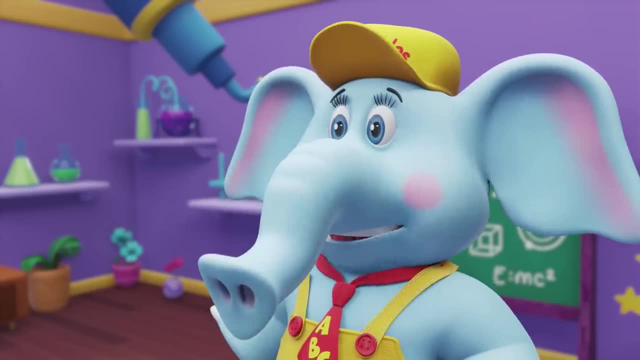 But we should probably stay inside Lionstein. can you take us back to that sunny day Right away?